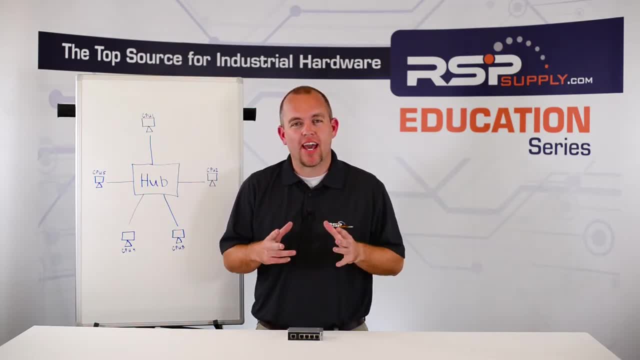 of the data being sent in any way. This can really bog down our network, because the hub is simply sending messages to every device connected to that hub. It also offers very little, if any, security for your network. It's because of these disadvantages that, in most cases, hubs have been replaced by network. 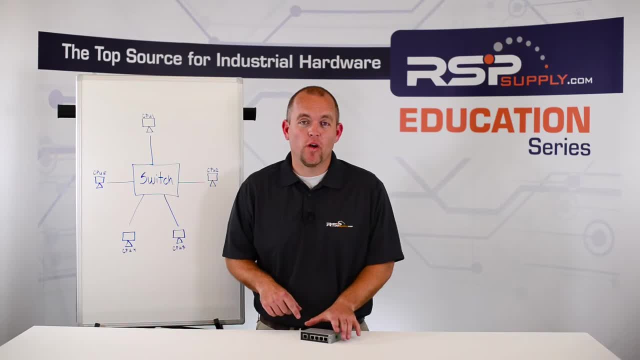 switches. Let's talk about switches Much like a hub. a switch, which we have here, is a device that is intended to transmit data from one device to another with any given network. Unlike a hub, a switch can learn where that message needs to go. 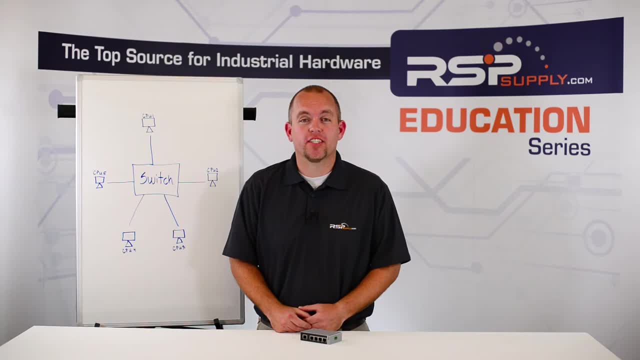 It can also learn where that message came from. It uses something called a switch table. The switch table stores which port a particular device is connected to. It also stores the MAC address like a physical address within a network of every device connected to that switch. 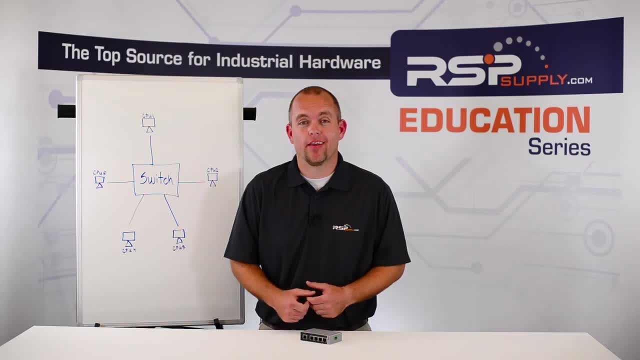 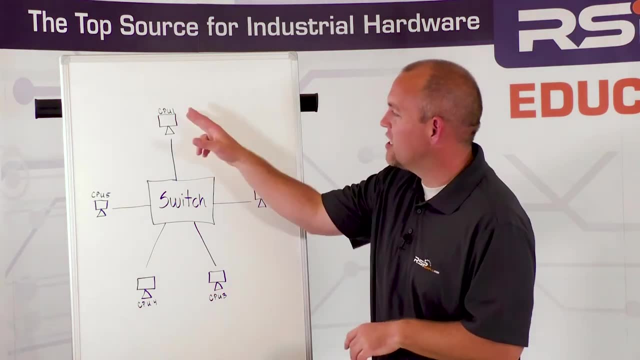 By storing this data, a switch can operate much more efficiently than a hub can. It also greatly reduces the traffic within the network. Let me demonstrate an example of how this works. In this scenario, CPU1 wants to send a message to CPU5.. 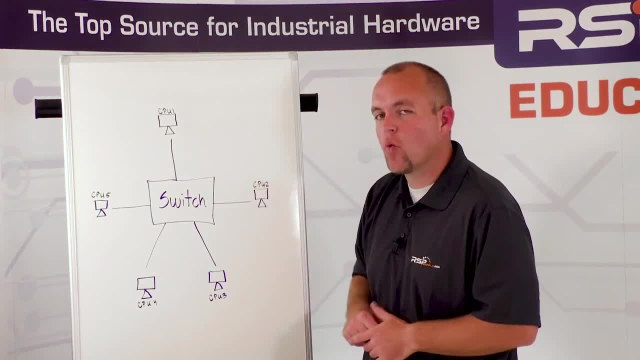 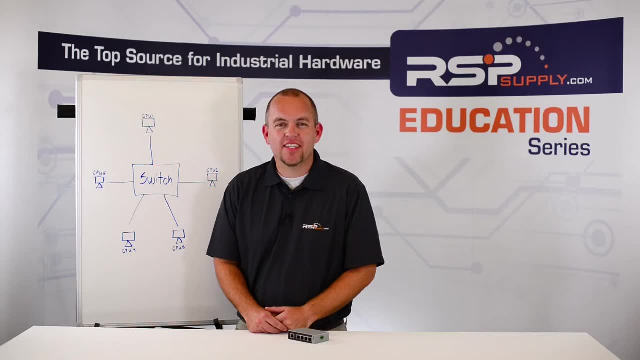 It sends that message through the switch. In this case, the switch knows where that message came from. The network has the opportunity to operate much more efficiently Because of these efficiencies. it allows data to be transferred between other network connected devices with less congestion. 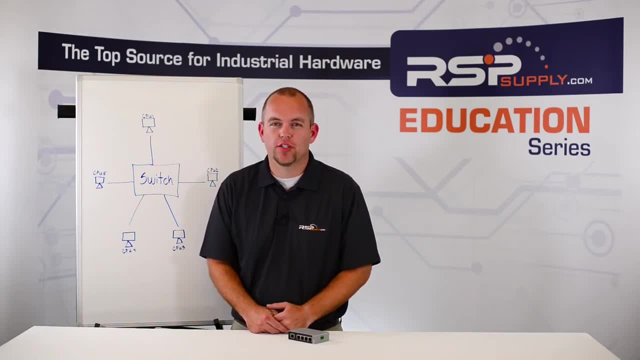 This makes the switch a great choice for almost all network solutions. The only disadvantage in comparison to the hub is cost, although the cost of switches has become very reasonable in recent years. Lastly, let's look at routers and what sets them apart from the other devices that we've. 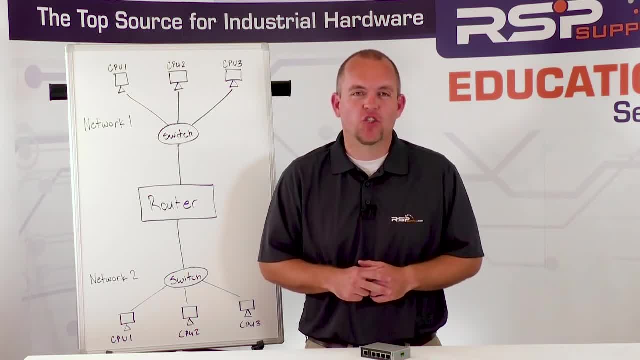 discussed today. Much like a network switch, a router can transfer data between devices while learning the location of those devices within the network. It also performs other very important tasks. It can act as a junction between two or more networks, as you can see here. 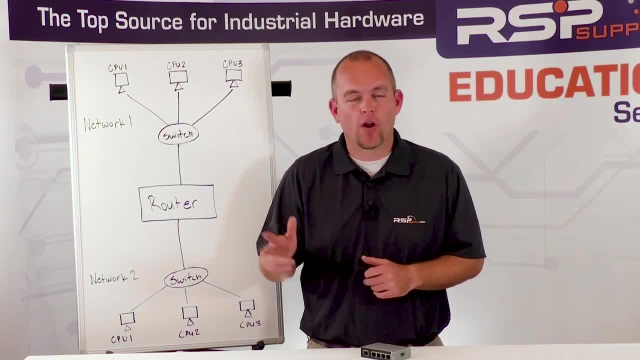 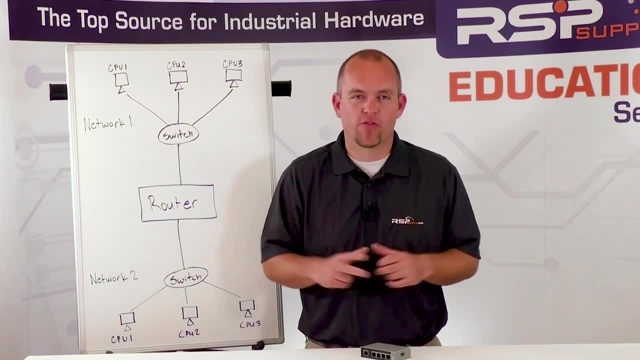 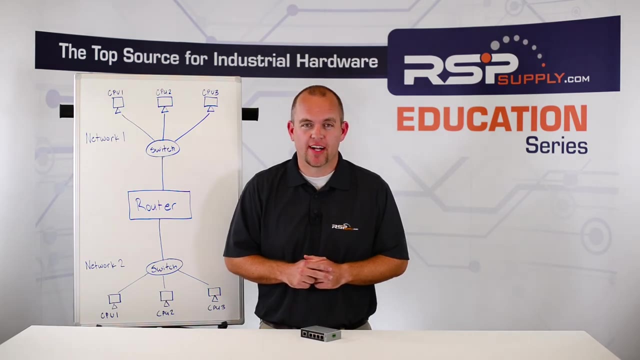 An example of this might be a home router in which the home network is connected to the internet. Another enterprise example might be when the router connects two or more networks with different business functions. In addition to connecting two or more networks, The router offers important security features that help protect our network.